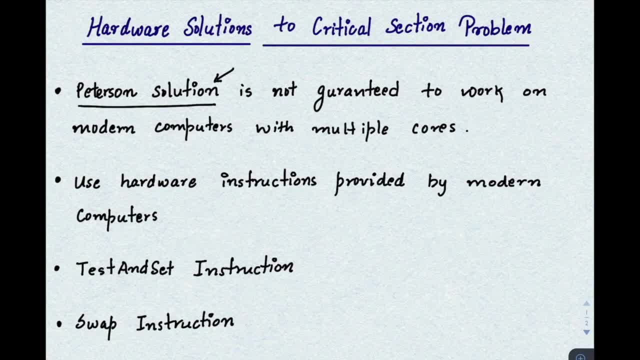 Peterson solution satisfy all the three requirements, that is, mutual exclusion, progress and bounded weight. but still Peter solution is not guaranteed to work on the modern computers which has multiple codes. so I've discussed the exact reason like why it is not able to work on the modern computers in a 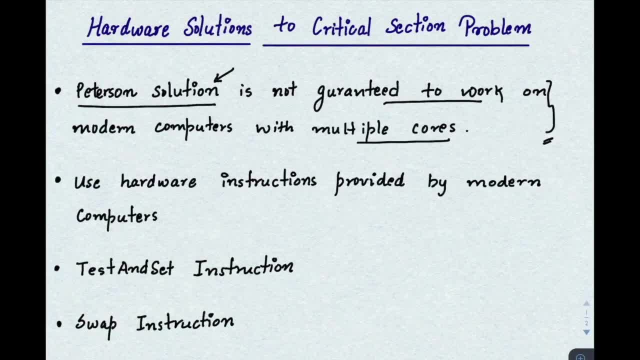 separate video. I'll attach that, the link of the video in description, so you can watch that and understand in details about this issue. now we will use some hardware instructions that is provided by the modern computers to solve the critical section problem. so we will look at the two instructions, that is. 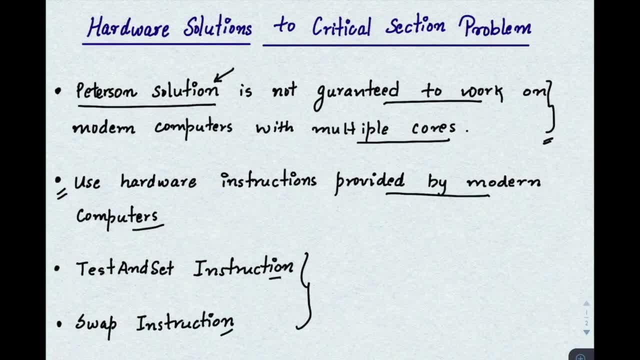 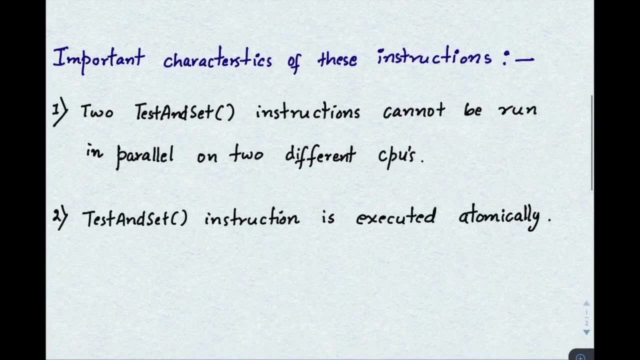 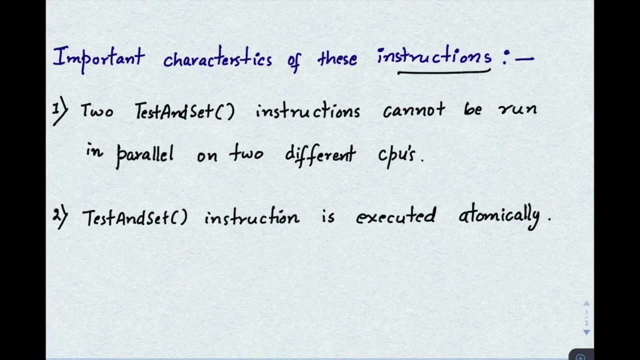 tested instruction and swap instruction, so both are hardware instructions. but before proceeding to these two instructions, we should remember two important characteristics of these instructions. so these two instructions are provided by the hardware, and also hardware guarantees two things. so the first one is that two test and set instructions cannot be run in parallel on two different. 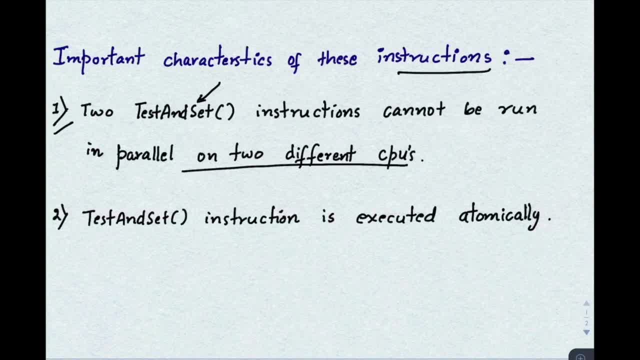 CPUs, so the only one test and set instruction can be run at a time, even if you have multiple processors, but Hardware will take care of, I mean care of running only one of these instructions. so let's see, even if you have two Threads, t1 and t2, and they both call this instruction- I mean test and set- at the 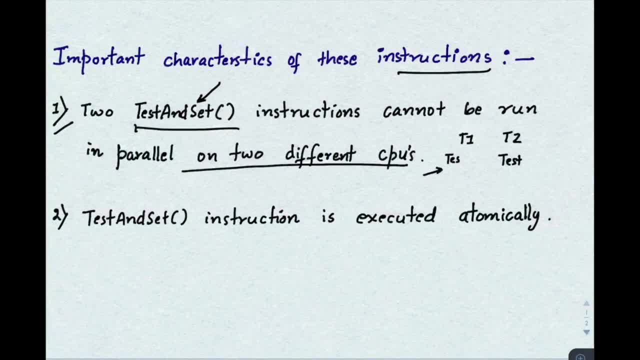 same time. even then the hardware will make sure that only one of this is able to run, run first, and once that, I mean once the instruction that was running completes, only after that the other can run. so both cannot run in parallel. and the second guarantee by the hardware is: 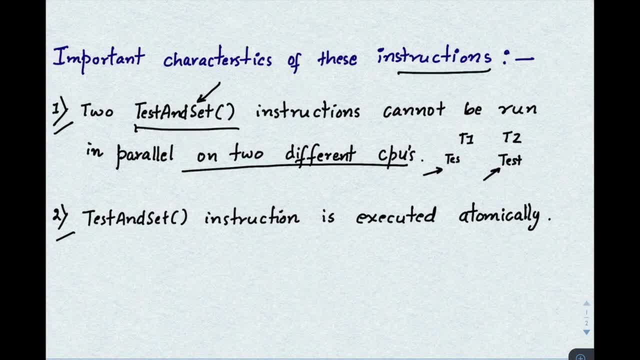 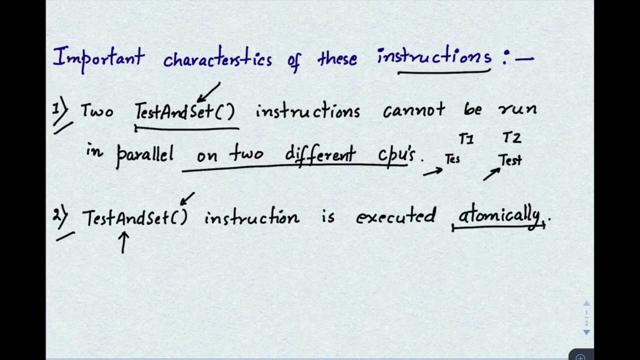 that the test and set instruction is executed atomically. so atomically in the sense that once this instruction starts executing it cannot be interrupted. it cannot be interrupted either by the hardware interrupts or the so so can also cannot schedule this process when this inclustcon is being driven. so that is guaranteed by the hardware itself. so if 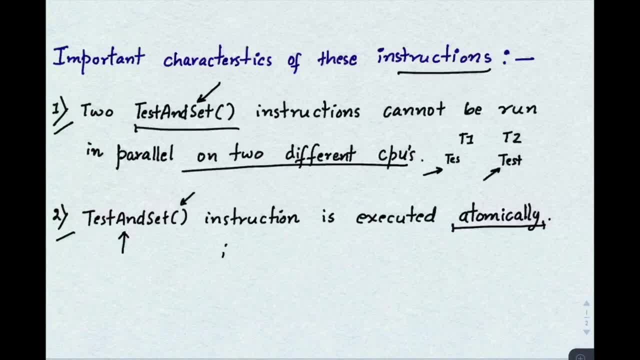 you remember, the main issue for the race condition was: first was the parallel execution. So if you have multiple codes and if you are trying to run the same code at, I mean that is shared so there will be some shared resource, And if you are trying to access that shared resource on multiple codes at the same time, 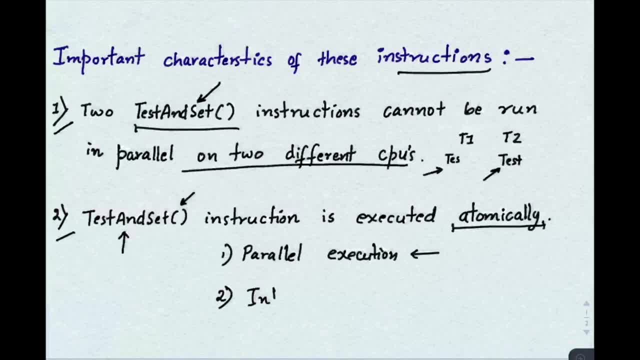 then the risk condition can happen. The second was the interrupts. Another reason for the risk condition was that when you were accessing the shared resource or when you were in the critical section, if it was interrupted by some hardware interrupt or the kernel said you are a reseller, then also the risk condition can happen. 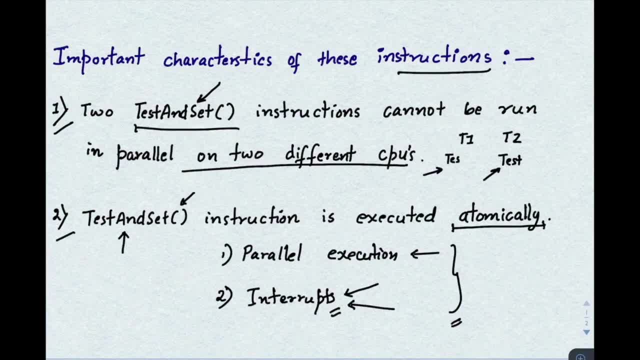 So I have already discussed about this when I was talking about the critical section and the risk condition, And here what we are doing is, with the help of hardware, we are trying to remove both of these issues that we had. So, since hardware guarantees that two same test and set instructions cannot be run in, 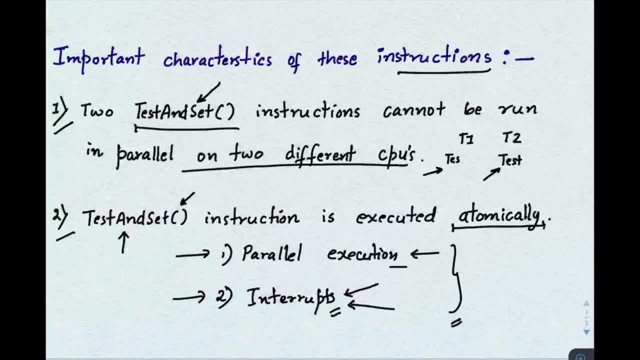 parallel. so we are guaranteed that this issue won't happen. And second is that it guarantees that it happens. this instruction, test and set, or the swap, is executed atomically. So now this issue also won't happen, because interrupts won't be able to interrupt this. 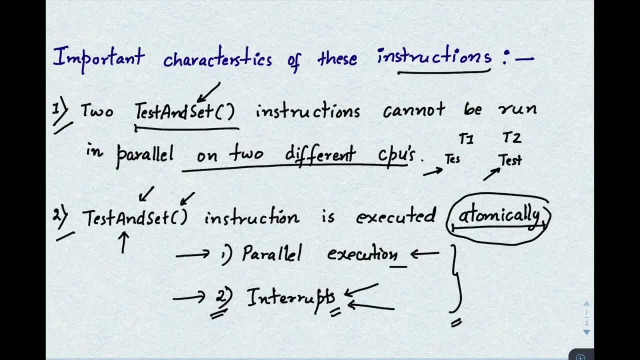 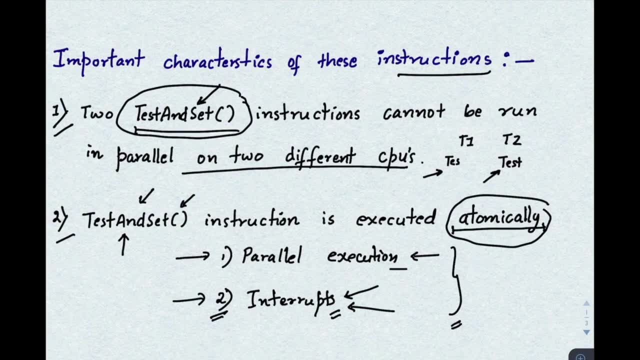 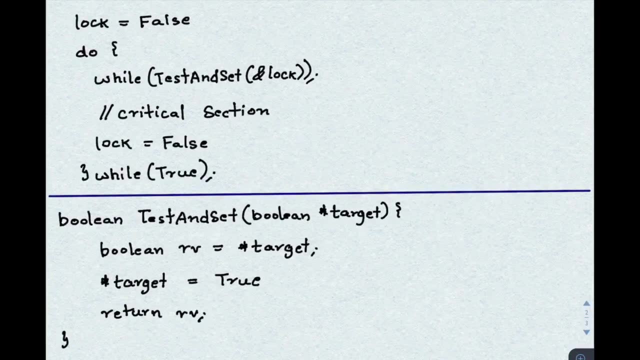 instruction. So now we will see test and set instruction like how we can use test and set instruction to solve the critical section problem. Let's now move to the solution based on test and set instruction. So this is the definition of the test and set instruction. 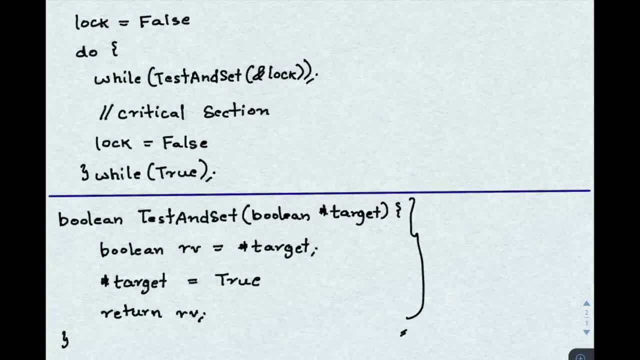 And this is guaranteed to be. I mean run by only one process or instead at a time, And also this whole three instructions will run, I mean without any interruption, Only after these three instructions have run. after this it can be interrupted, but not. 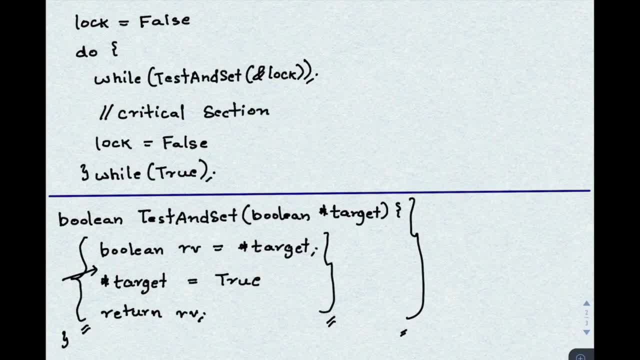 in between this, So you won't have an issue of race condition within this instruction itself. That is guaranteed by the hardware. Now you will see that what this instruction actually does. So what it does is it actually takes a target, and you have to remember that this is a pointer. 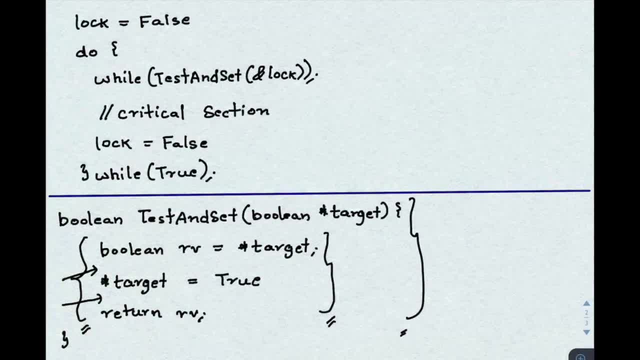 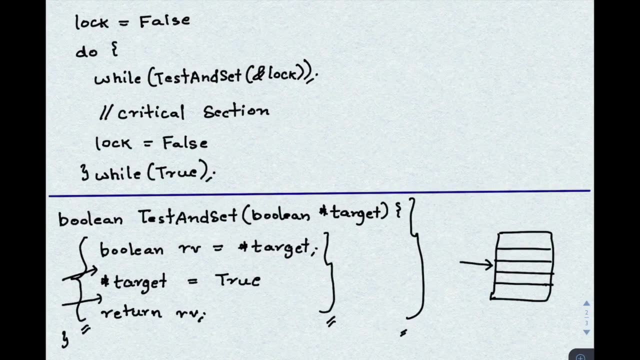 actually So. pointer is actually so. pointer only stores the memory address. So you will have the RAM and you have different memory addresses and this target just points to one of this. So this: so this will have some address right, So this target stores the address of that. 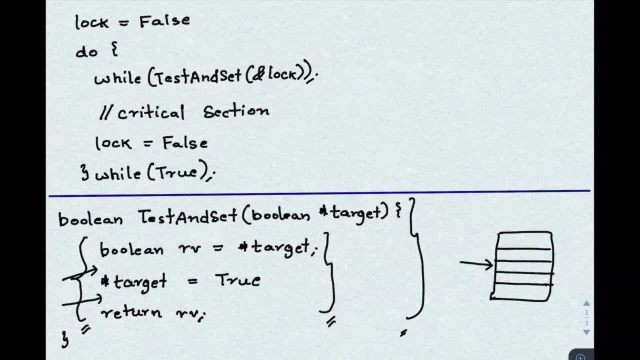 Now, What you're doing is So when you write it as start- so start target, I mean start any PTR- it gives you the value that is stored in this address. So what you're first doing is we are storing some return value that we will return and 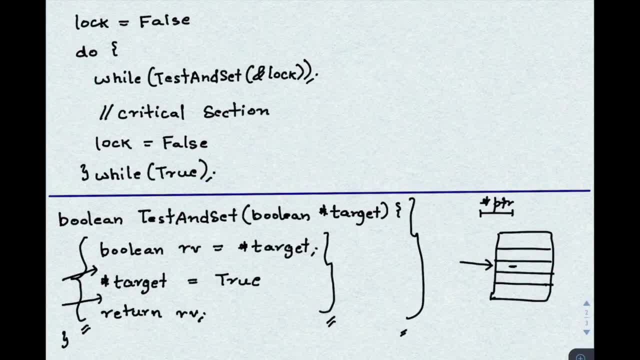 that is start target, So that is the value that is stored in this memory address. Then we are setting this, So this is a target here, right Now. we are setting this to true And then we are returning the RV. That is the value we have stored right. 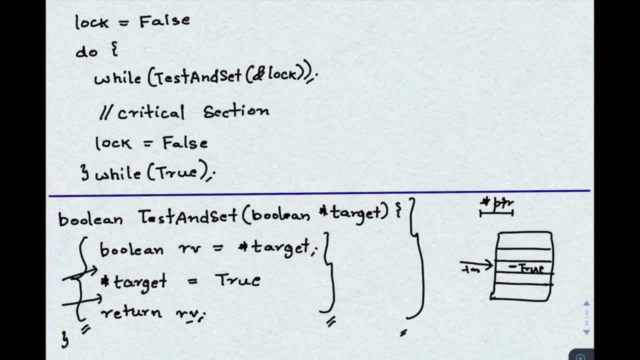 Think of this case, when target is either true or false, right. So we will see the output of this test and set. So let's say, when the output- I mean when the boolean start- target, it is true, right, The input is true, right. 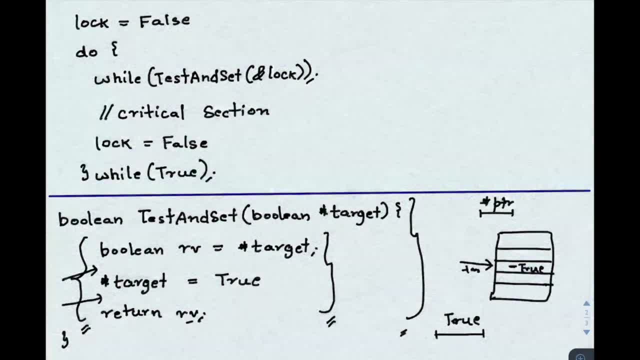 So what will be the output of this code? So what it does is it returns the old value. that is there, right. So what it does is It replaces the old value. It replaces the old value with true and returns the old value. 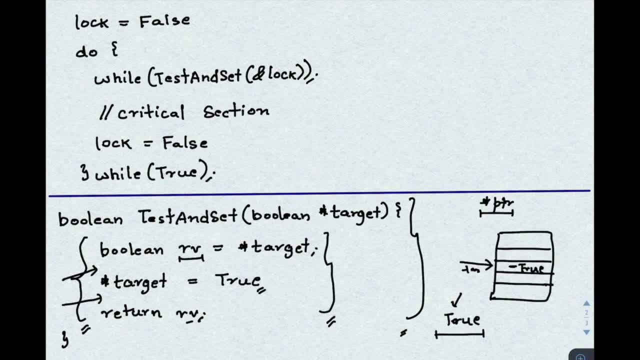 So here the old value is true, So it will again store true in this, where we just replace true by true and then return the output as true. But when the target is false, let's take that also. In this case it will store this in return value that is false. 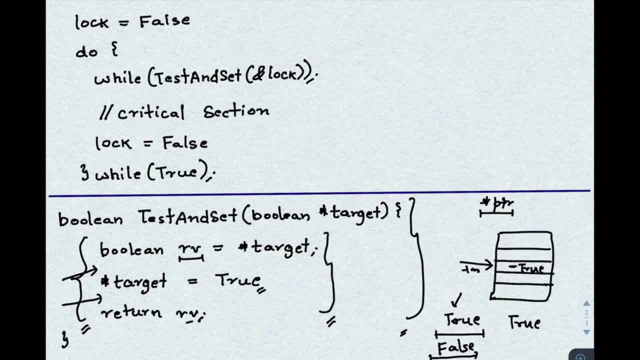 Then in target it will make it as true. If it is false, the target will be true. So in memory: initially it was false. right here it was false. Now this will be made true and it will return the old value, right. 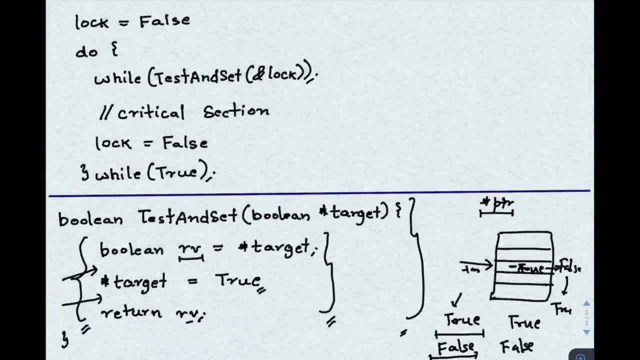 So that is false. So it's simple: When you give the input as true, it returns true. When you give the value as false, it gives false. But there is one difference here: It also says the value of target as true. 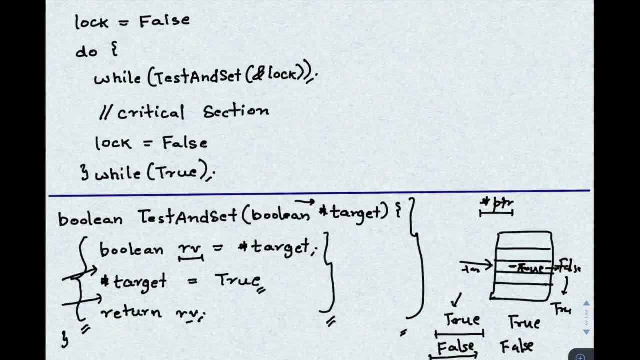 And since it is passed by reference, Or if you see here, it is passed by reference, right. So this value target will be changed in the memory itself. Now let's look at the. this is the critical section code for mutual exclusion. 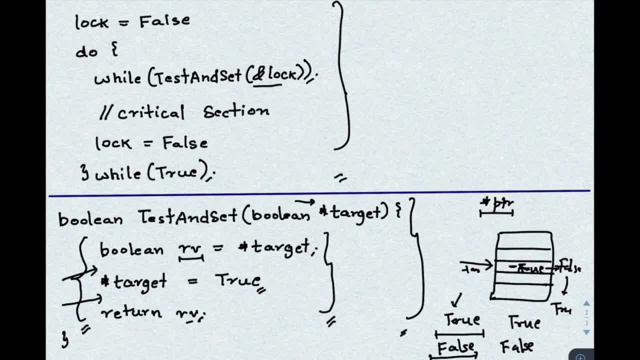 Now let's look at this code. So now we have a log variable here that is set to false initially, And this will be shared by, let's say, all the threads which are there. Now what you're doing is, while, test and set. 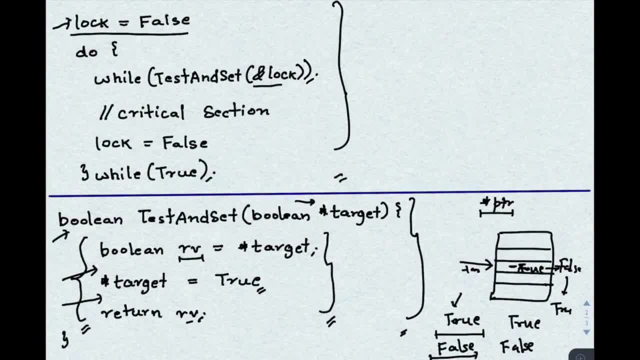 And you're passing this log to this function that is described here and you're passing it by reference, right? So any changes that is made to this will be reflected in the memory. So here, target right. If you change it to false or true, here it will be reflected in log. 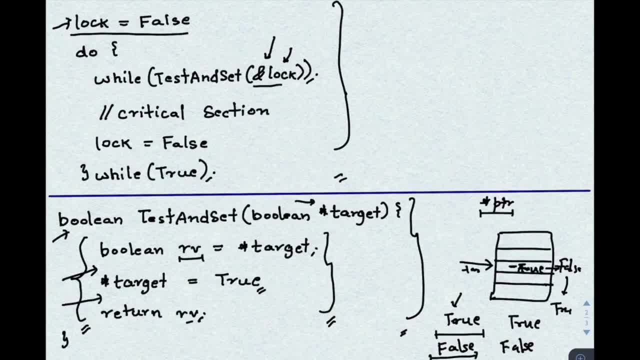 So if you change the target through here, then log will be changed to true here, since it is passed by reference. So okay, now see what will happen. Let's say there is a process. I mean, let's say process, This is P1 that arrives first. let's say you will take the case when P1 and P2 arrive. 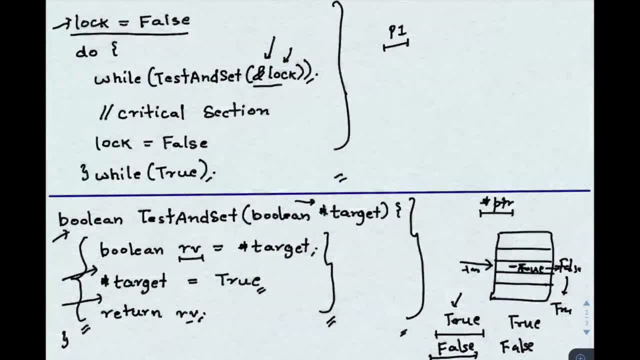 at the same time. but let's take the case when P1 arrives first, then log is false, right, And this test and set log what this will return. since the input here of log is false, it will return false And this while loop will break. 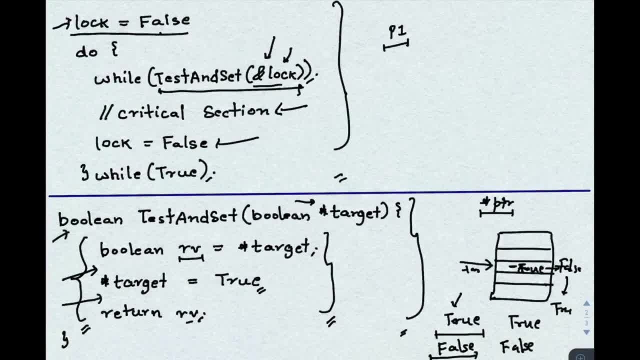 Now it will go into the critical section And finally in the exit section. so this is the entry section here. this is the exit section. it will turn the log as false. Then it will exit. right, Let's check the case. 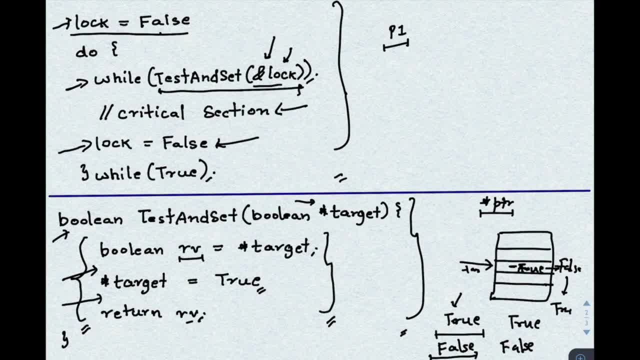 Okay, now we will describe. okay, I think you would have understood the solution here, right? So this just returns false and this enters right. But let's say when it was in critical section. this P1 was in critical section, remember. 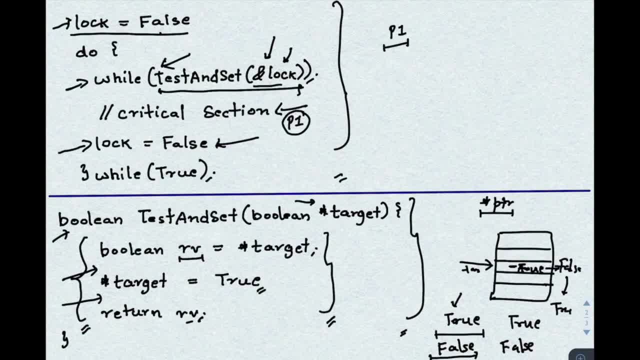 that the value returned here is false. but in this code the target has been set as true, So that is log itself right, Since it was passed by reference. So the value returned by this function is false, So that is log itself right. 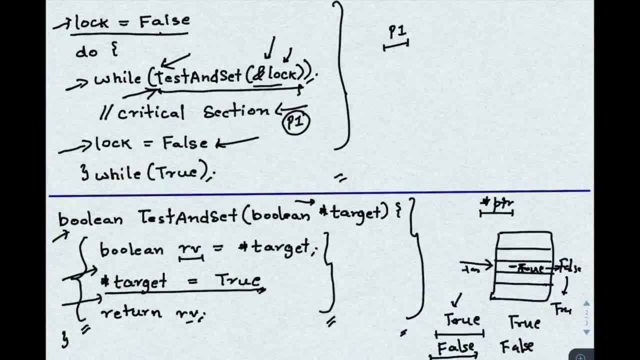 So the value returned by this function is false but the value of log is true. So when P2, so now P1- is in the critical section and P2 wants to enter this, so first it has to go through this while loop and it will check. while test and set again, it will check. 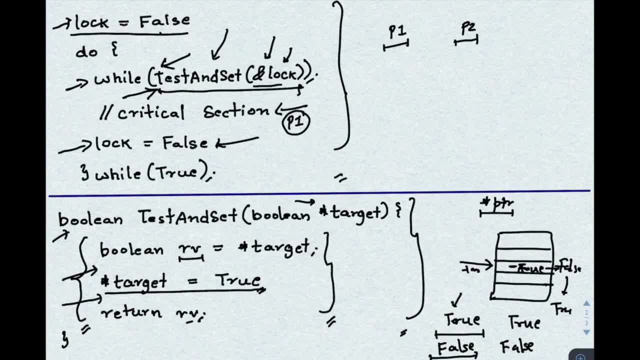 this. but now the value of log is true, So it will go in this and we know that if the value is true, it returns true, So this will while true. so it will be stuck in this while loop only when the log will. 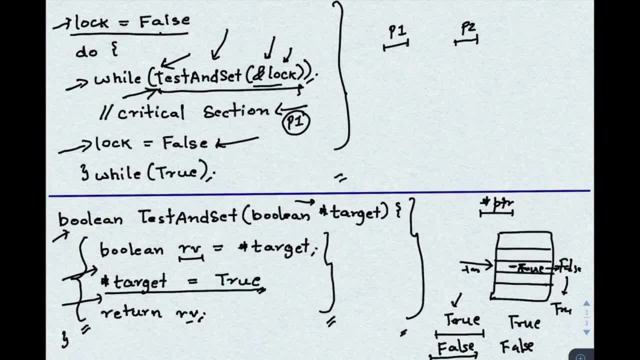 be made false, Then only Then, only Then, only So once again, when it tries again, then it will return false there, then it can enter right. So let's consider now case first of mutual exclusion, how it satisfies mutual exclusion. 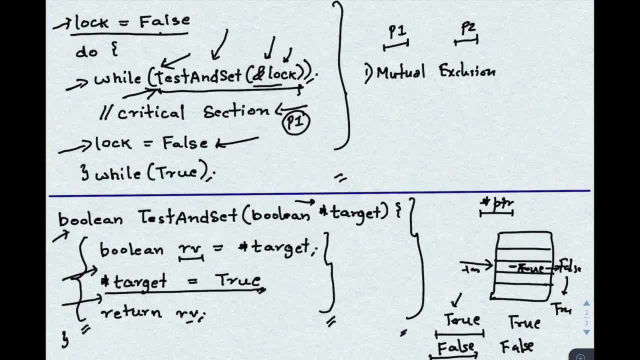 We will look at all the three. So if you, if you remember what I have told is that test and set, if, even if P1 and P2 tries to enter here at the same time and execute this instruction, test and set and the log. 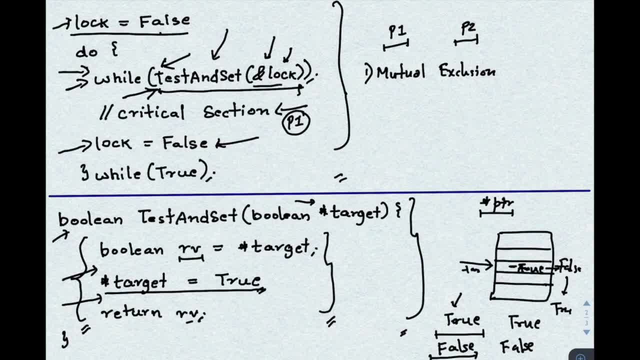 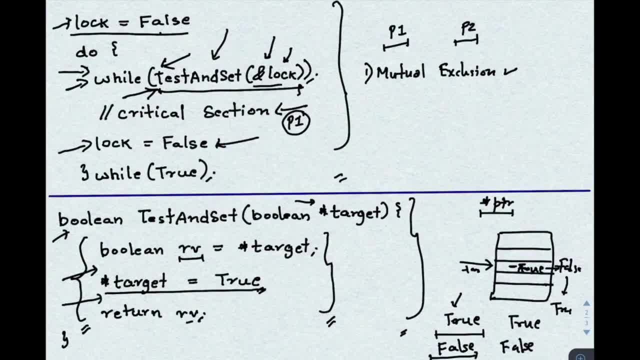 mutual solution will be here, because this, this will. I mean, let's say, if p1 was able to run this instruction, then p1 will be able to enter. if p2 was able to run this section, then p2 will be able to enter the critical section. but it is guaranteed by the hardware that p1 and p2 cannot run this. 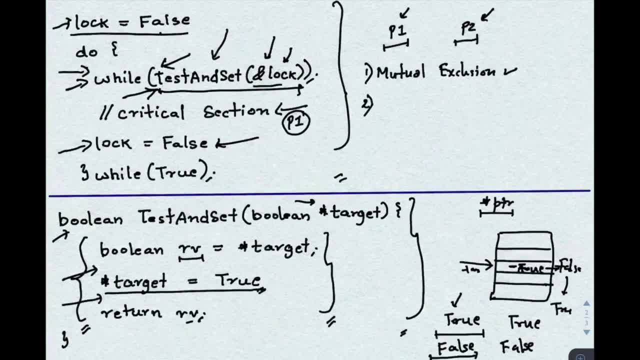 structure at the same time. now let's go to progress requirement and also deadlock cannot happen here because- and since you have already have, I mean it is guaranteed by the hardware that this can be only run by one process at a time. so I mean deadlock, you will. 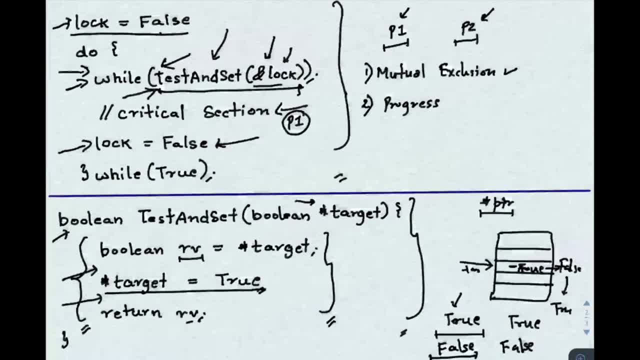 have when both tries to execute this at the same time. but that won't happen in this case as it is guided by the hardware. so deadlock won't happen. and if you think about progress here, so what you can do is, let's say, one process, process p1- it is able to acquire the lock, then it 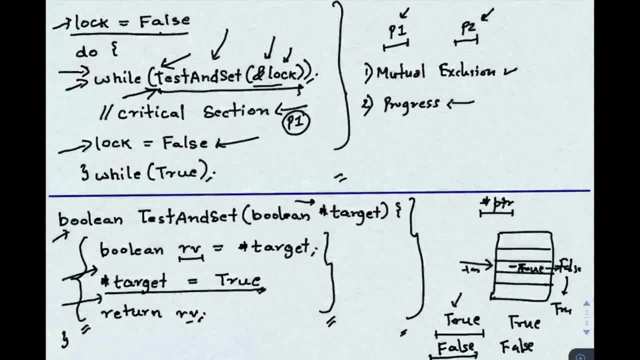 makes the lock as false, then it exits this. and now p1 does not want to, I mean doesn't want to enter into the critical section, it wants to sleep. let's say after this: it does not want to enter from here, it just wants to sleep. let's say right. and now let's say p2 wants to enter. right now p2. 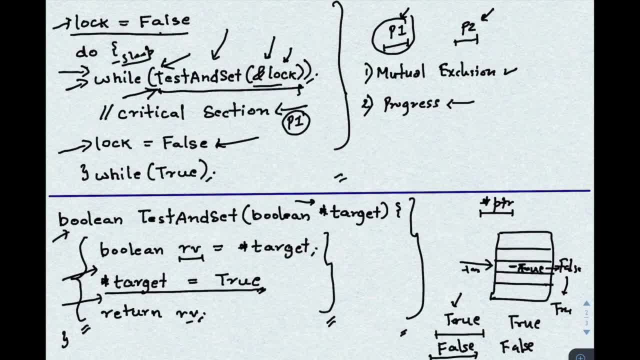 the p1 has- I mean exited from this, then the lock will be false and p2 will get the access right. and again when it tries to- let's say, for the second time, it tries to go into this restriction again, it can go again right, because while exiting it will say the lock is false. 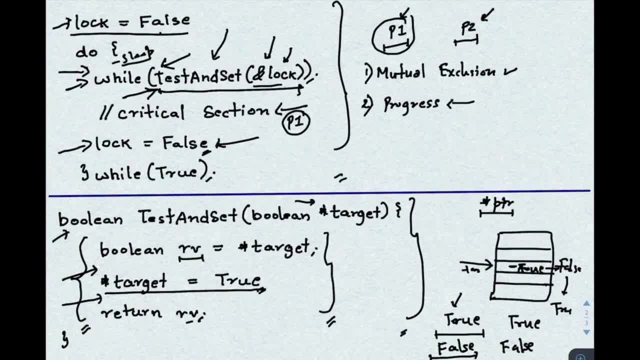 and again, since lock is false, the value written from this will be false again. it can enter. so it's. it's not here that if p1- I mean p1- cannot block p2 from entering, even if p1 does not want to enter the critical section. 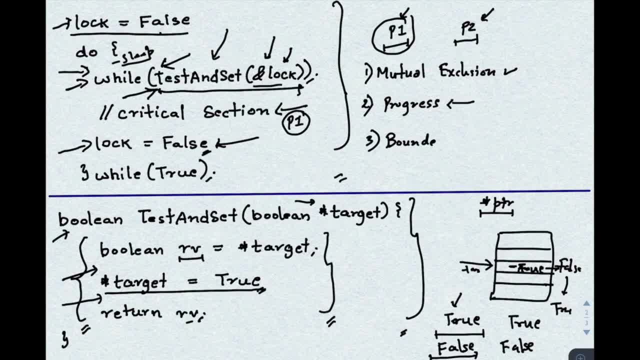 third is bounded weight, so bounded weight is not guaranteed in this case. I will explain the reason. so if you see this while loop right now, take this example: if p1 has already gone into this critical section and it is trying to enter again and p2 was also waiting at this while loop, so p1 is trying 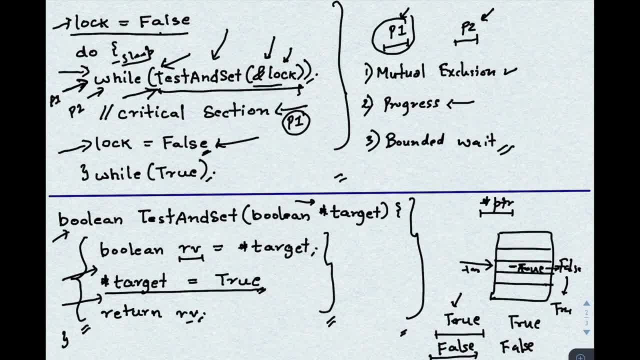 to enter again and p2 was waiting from before, also right, but there is no way that- I mean there is no way- to block p1 from entry again, right? so p1 and p2 are again trying to. I mean, they are racing for this instruction and we already know that this will be executed by 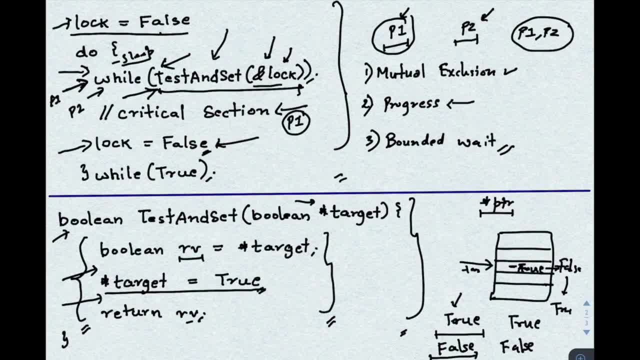 one of them. so hardware only guarantees that only p1 or p2 will execute the instruction, but but it does not guarantee the order in which that will happen. so it can again happen that p1 will get the access to run this instruction and again when it is- I mean again it wants to. 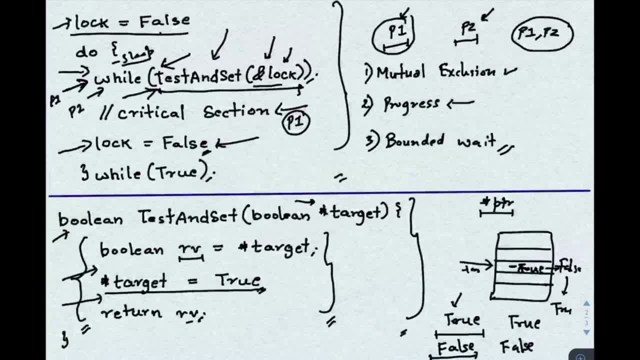 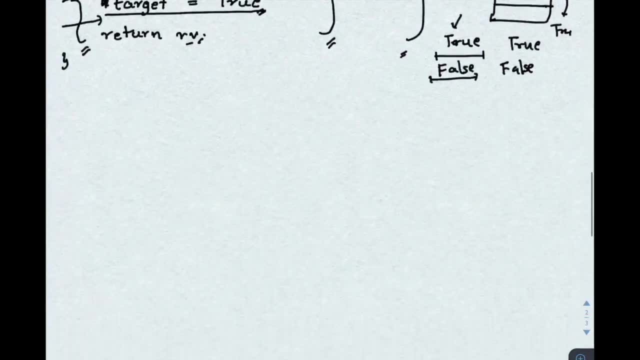 run, it can again do so. so there is nothing stopping p1 from not entering, I mean like intersection again, or not entering this while loop itself right. so that's why boundary weight is not satisfied here, and so if you, if you look at the drawbacks of this, so I will say that first.